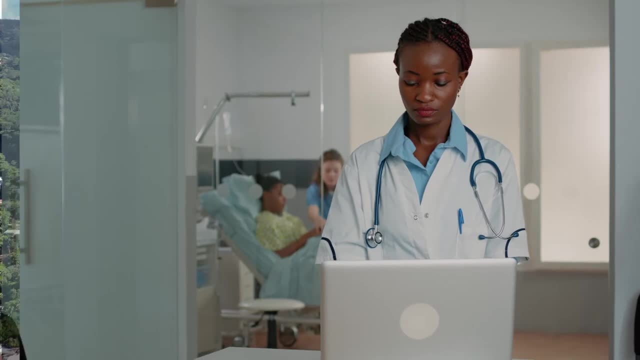 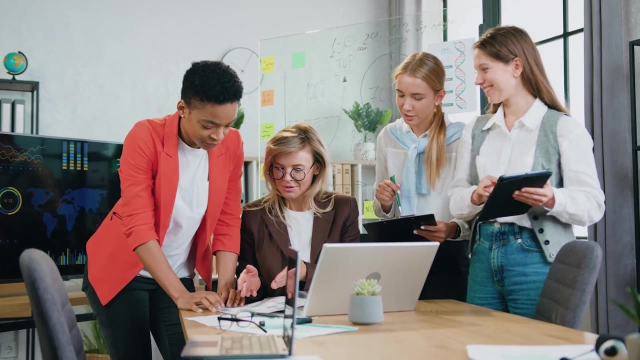 population's NIR. you can see that they have a higher NIR. As societies develop, gain access to more modern medicines, continue to urbanize and provide more opportunities for people to participate in the society, they start to see their growth rate slow Historically. 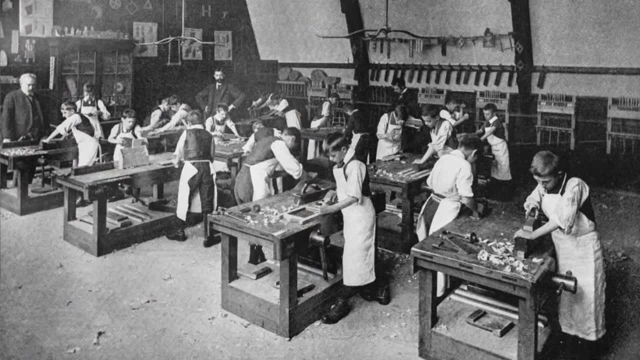 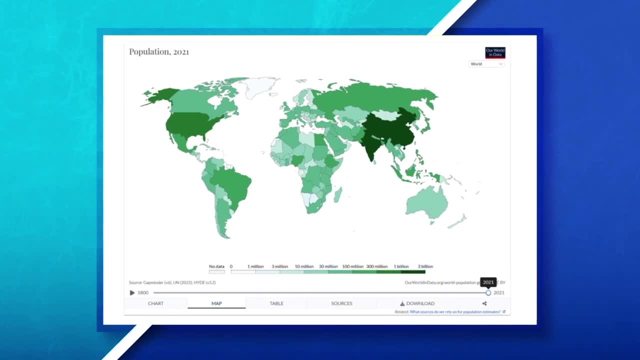 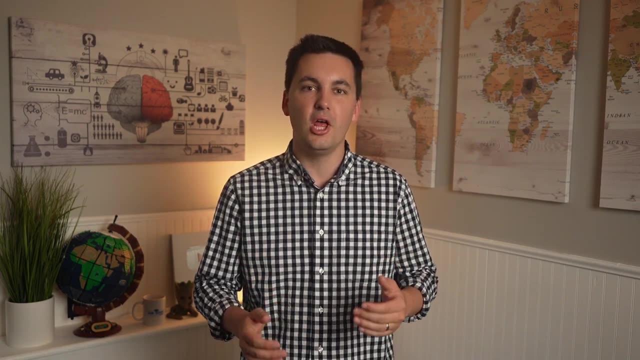 events such as the industrial revolution and medical revolution led to population boom, As societies started to see a higher life expectancy and lower infant mortality rate. Today, we can see that population dynamics are heavily influenced by a variety of different social, cultural, political and economic factors. Social factors, such as investment. 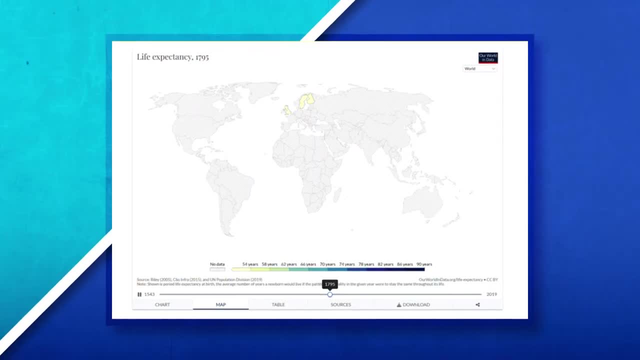 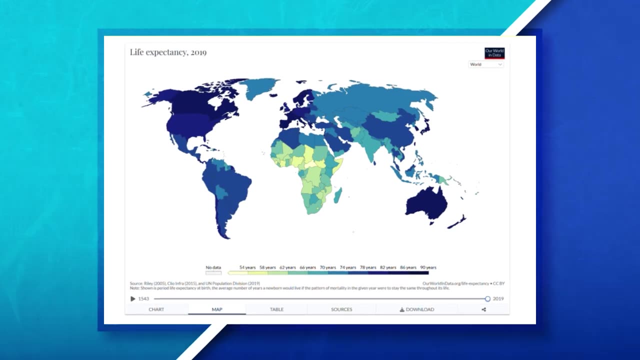 in health care and education allow for a society's life expectancy to increase while at the same time can also decrease a society's total fertility rate and infant mortality rate. When a society promotes education for men and women, they often see their TFR decrease. 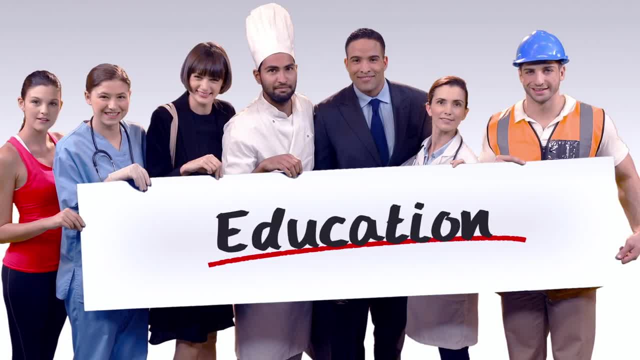 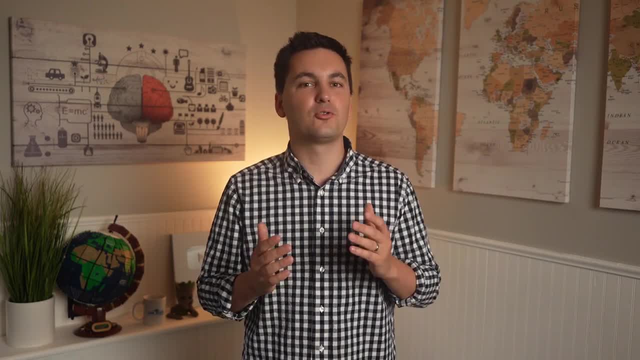 This is because, as more people get an education, they gain new skills and abilities that allow them to participate in the workforce, which pushes back a person's timeline for having a better future. If we look at a society's cultural values, we can examine how a society 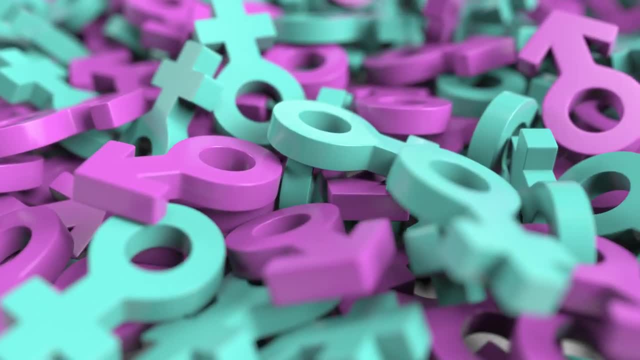 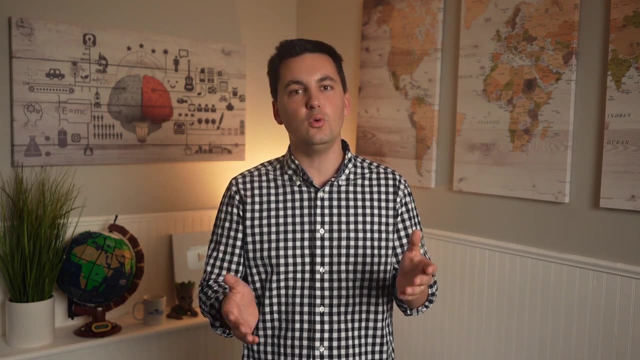 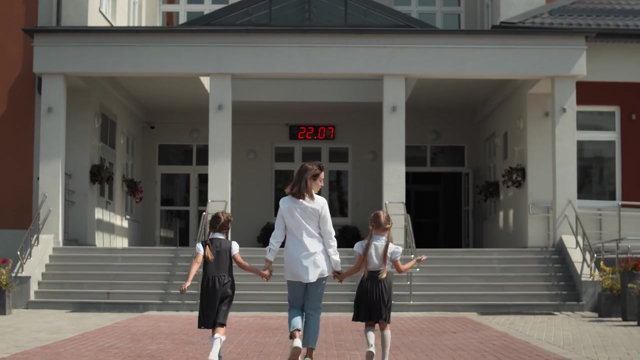 views the different sexes and what gender roles are established and promoted within a society. Societies that do not allow women to participate in the economy, attend school and view individuals with traditional gender roles tend to have higher TFRs and a higher NIR, But cultures that open up more opportunities for women in school, society and the economy. 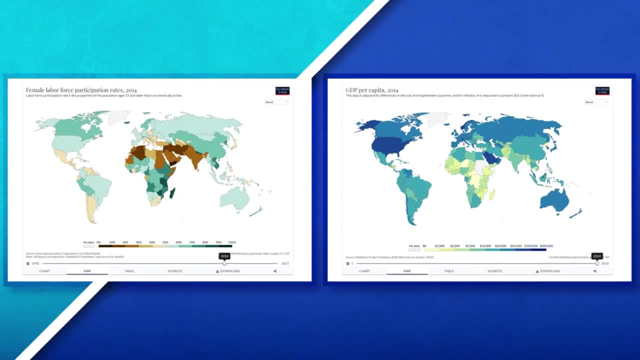 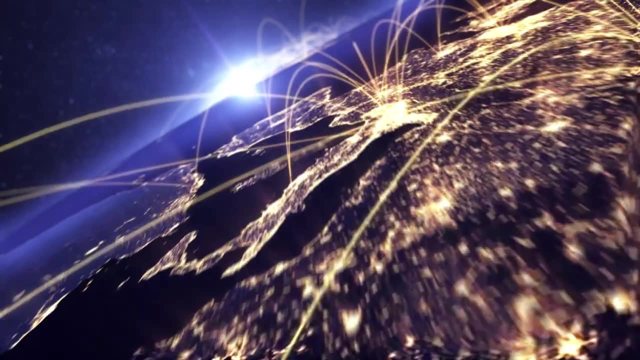 tend to see their economies grow, their TFR decrease and their NIRs increase. The reason why women are more likely to participate in the workforce is because they have a higher NIR and their natural increase rate level out. As societies develop economically and become more connected to the global community, they often see their cultures shift As people. 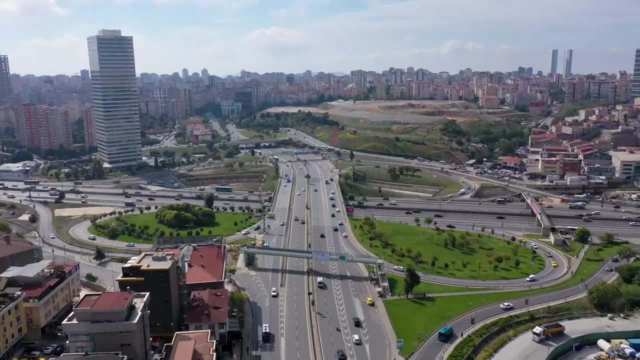 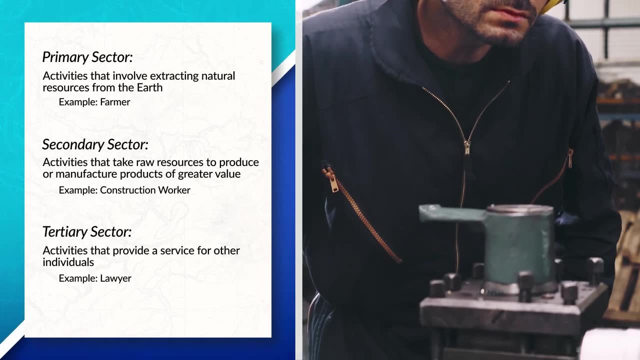 become more aware of other cultures around the world. as societies grow and develop, we start to see more people moving to urban areas. Jobs start to shift out of the primary and secondary sector of the economy and move into the tertiary sector. These economic changes. 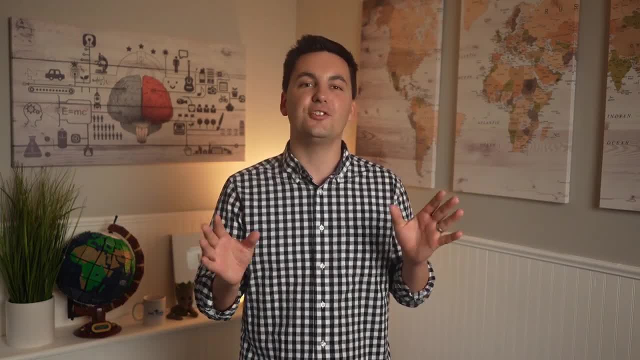 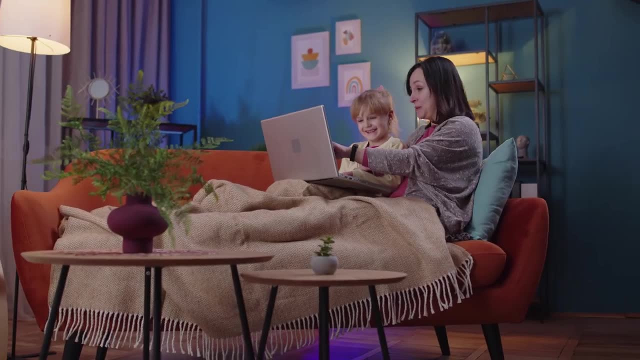 influence a society's culture, birth rates and the day-to-day lives of everyday people. Developed economies with high rates of urbanization will often see smaller family sizes, since there's more of a focus on starting a career and less of a need for a larger family Family.